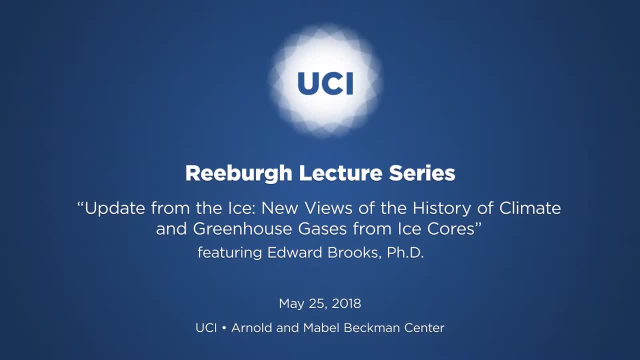 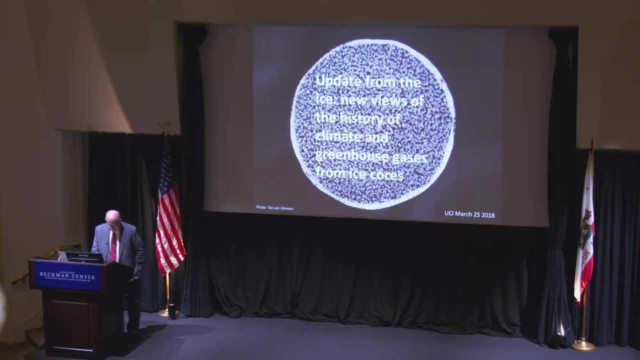 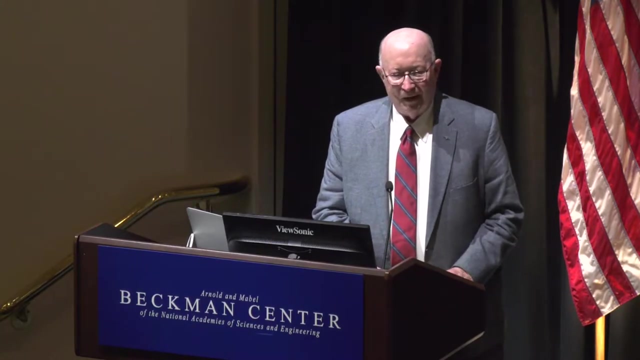 This lecture has grown and this I think we started off. this will be the sixth of the series annual lectures. The first one was held in the Crow Hall, the circular Jenkins room, and it turned out the very first one. the people were too deep around the circumference. 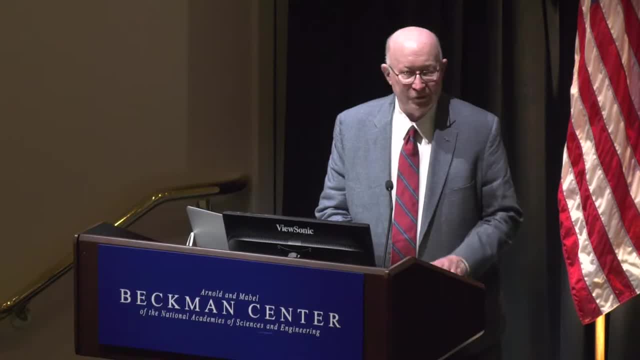 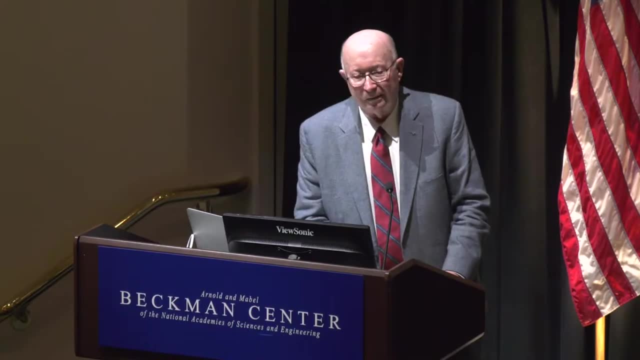 standing too deep around the circumference of the thing. I was one of the ones standing and it turns out that we knew immediately we had to change venue. So we switched and went to the Cal IT Square Auditorium and the first one that we had there was quite. 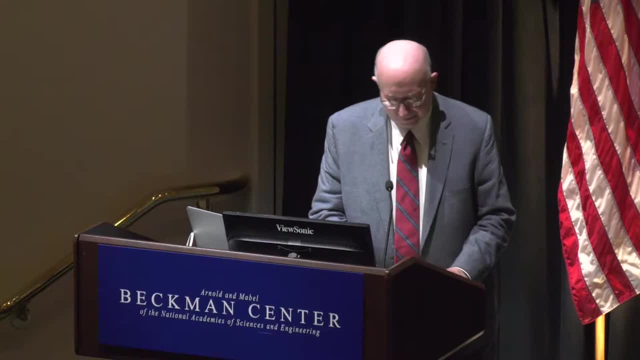 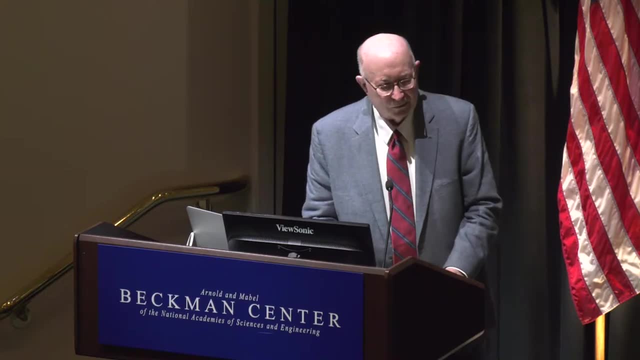 comfortable. The seats were vacant seats and it wasn't crowded and you weren't crunched up against your neighbor, and so that worked pretty well. but for the next two it grew and grew, to where, last year, the report? well, I didn't make the one last year, but 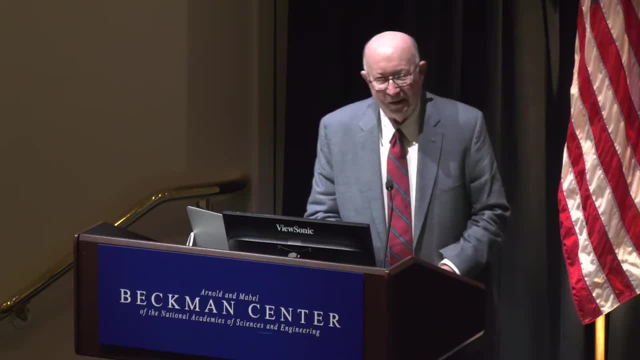 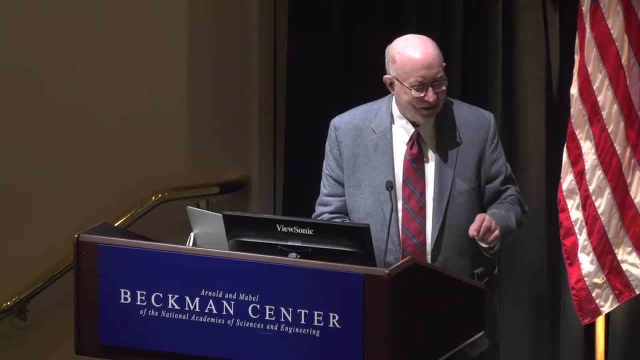 the report to me was that it was standing room only and there wasn't enough food, and the reason for that, apparently, was the fact that the standers ate the snacks and helped themselves while the lecture was going on. So it's grown immensely and I think that 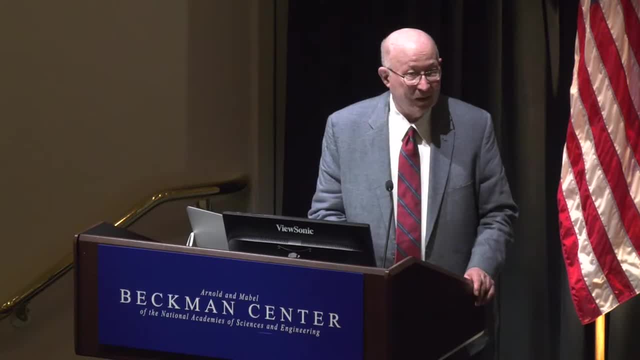 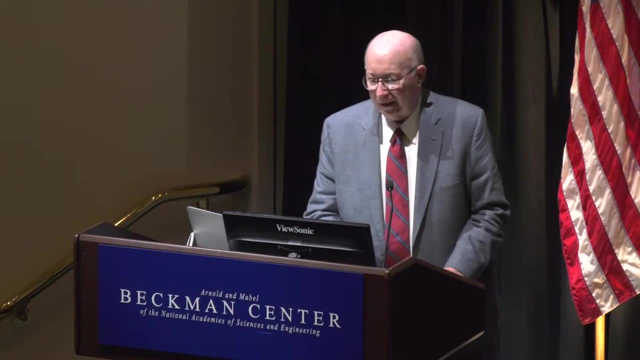 we're going to try to stick with this venue. It's a very nice auditorium. We all know that It can handle more people and it's going to be, I think, a real thing to look forward to in the future. One thing I wanted to point out, too, is that all of the previous lectures 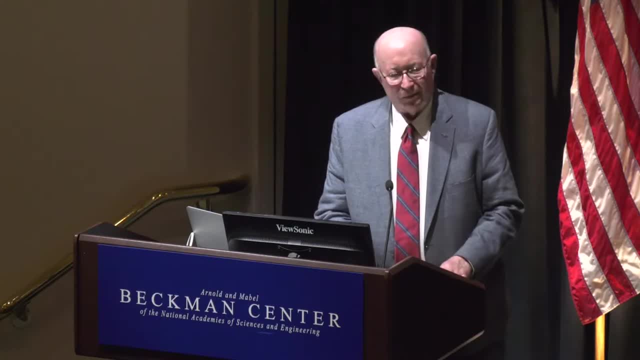 are on the department website. You go to the ESS website and go to Rehberg Lecture Archive and the previous lectures are there and if you want to see that, if you want to check this or pass the information on to a friend, feel free to do so. This I wanted to say 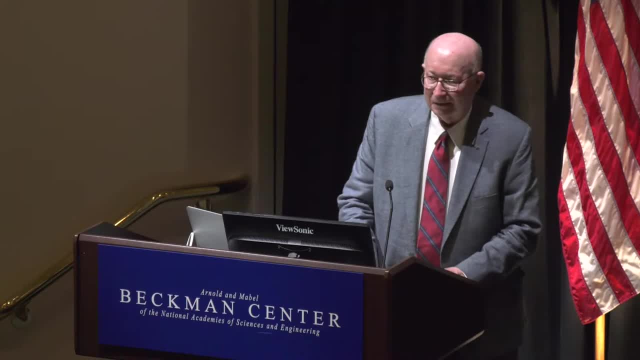 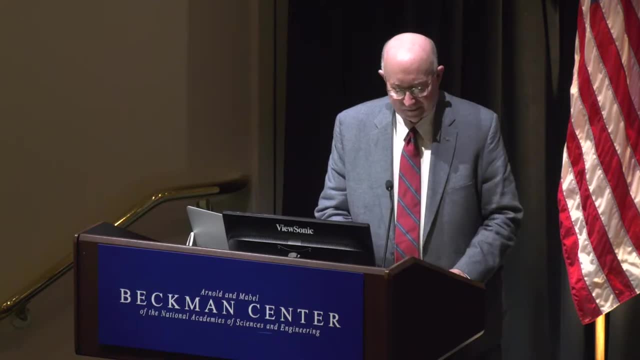 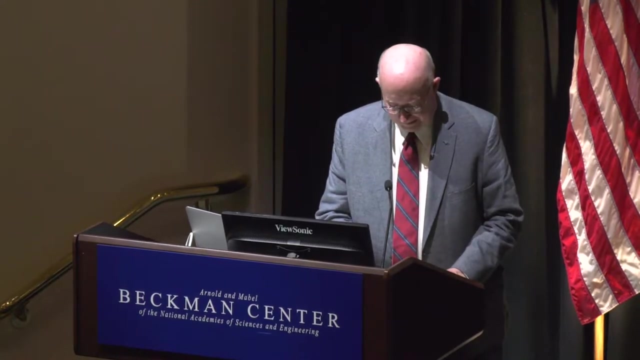 too, that the terminal disease that afflicted Carolyn and eventually took her from us last October was a kind of a thing. Well, like I say, I think that this lecture series is a really fitting tribute to her, her curiosity, her love of learning and her basically general attitude, and I think that 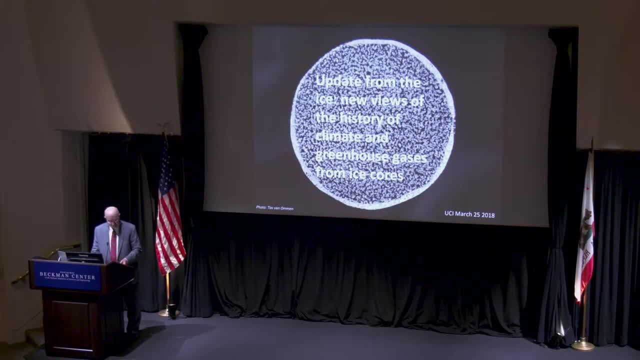 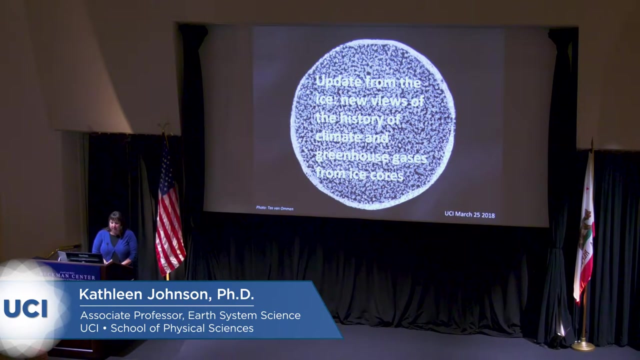 she would be very happy to be part of this. have her name on the list, the first name on the title of the lecture. So with that I'm going to bail. call Kathleen to introduce us. Hi everyone, So it's my honor to introduce this year's Carolyn and William Rehberg Endowed. 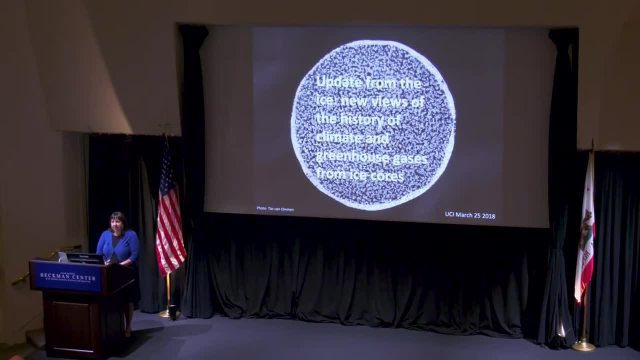 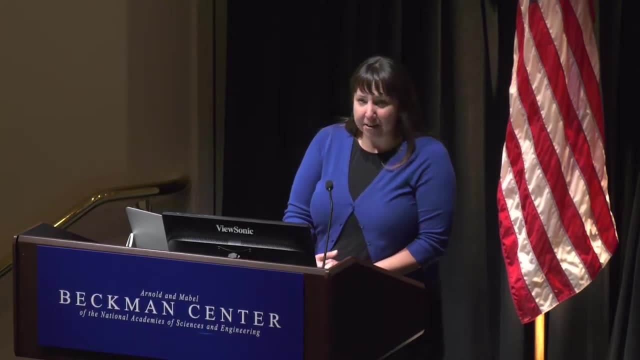 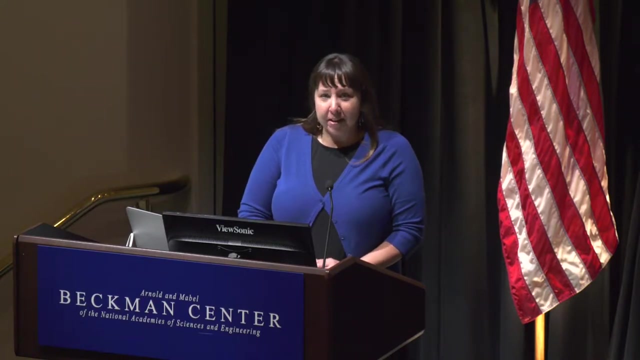 Earth System Science Lecturer. This lecture is traditionally selected each year by two research groups in the Earth System Science Department, and this year the honor fell to Eric Saltzman's group and my own, and we actually put quite a lot of thought into 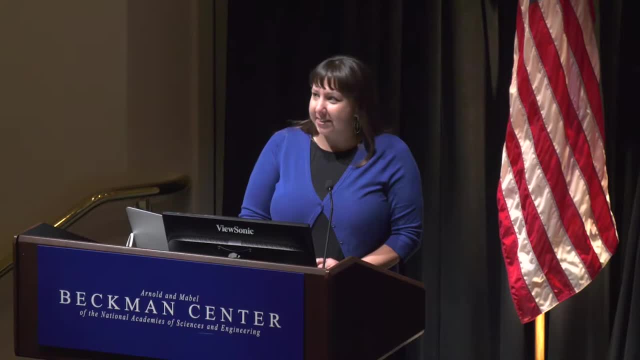 this process And we met a couple of times. we worked together with all of our students and researchers and we decided 100% democratically who to invite, And so I'm very pleased to introduce Ed Brook, who we selected to be this year's lecturer, As research combines fieldwork in 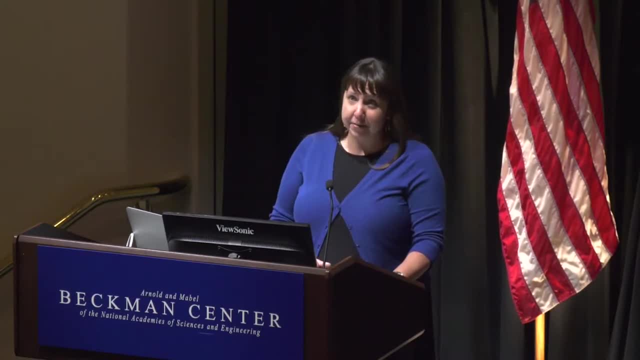 polar regions with very detailed and difficult analytical work in the laboratory to investigate the history of greenhouse gases and climate. And I'm glad for the wonderful go And it's a great honor to be here with you. It's a great honor to be here with you. 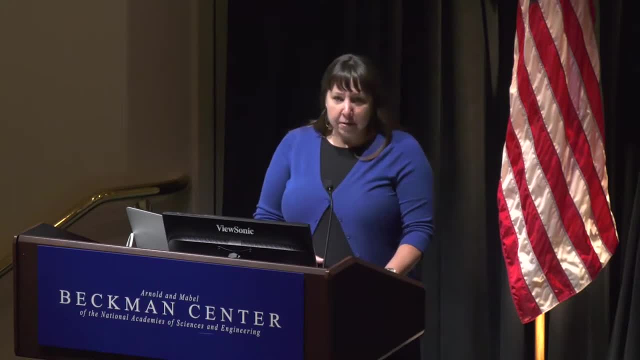 So first of all, I just want to thank ourertu and William for helping me with this talk. We've got some great stories to share, So I'm going to start off with a comment. So you didn't know about the, I'll just kind of pass it over here. 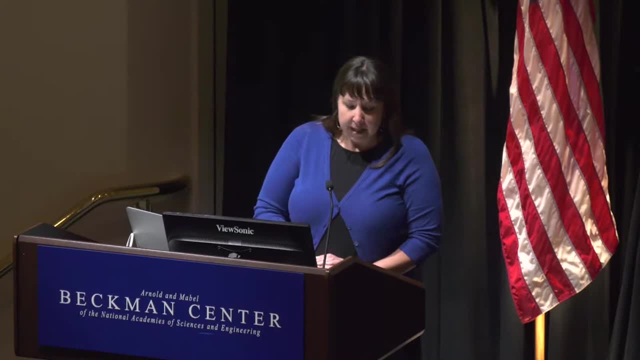 Thank you. So it's an interesting topic to get into, but part of the reason why I'm so looking forward to this talk is that we have a lot of important questions on the topic. Some of those have actually already been brought up in the chat, and I do want to include some. 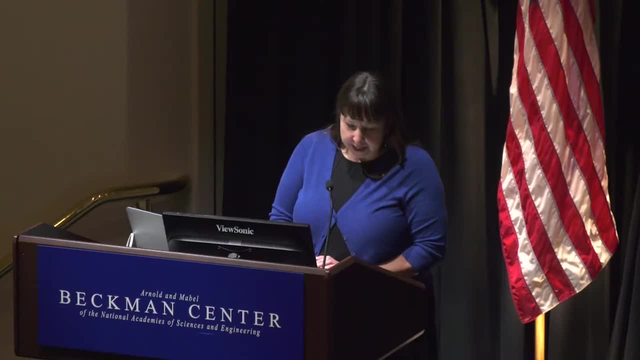 of them. So I've got a lot of questions about the topic, which we'll probably hear a little bit about today. And, of course, this topic is also highly fitting for the Reberg lecture because, given the huge impact that Bill's work has, 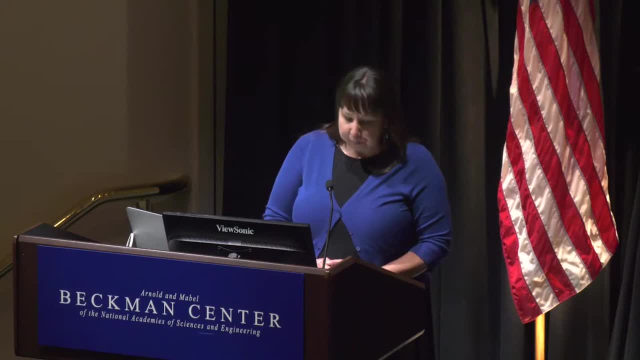 had on our understanding of global methane biogeochemistry. So, without further ado, I'd like to introduce Ed Brook. Ed is currently a professor in the College of Earth, Ocean and Atmospheric Sciences at Oregon State University. He was recently named a distinguished professor. 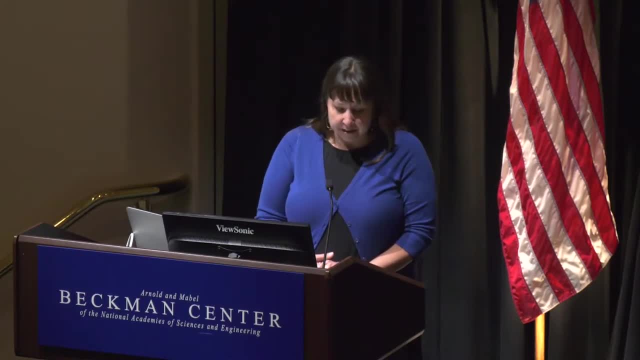 in that university, which is a select honor reserved for only a few people. He's also received many other honors in his life, including being, a few years back, elected as a fellow of the American Geophysical Union. He did his undergraduate and master's degrees in geology. 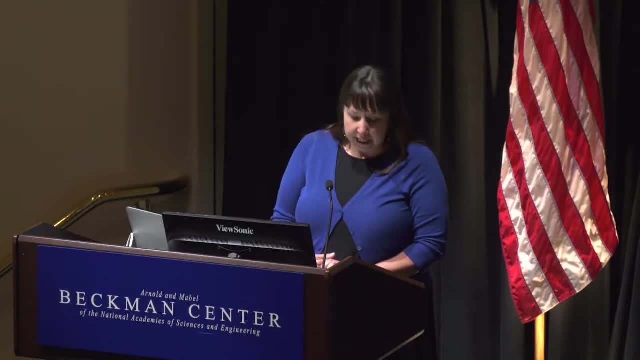 at Duke University and the University of Montana respectively, And then he did his PhD in chemical oceanography in the MIT Woods Hole Oceanographic Institution. So just one final word of thanks to Bill Reberg and to Carolyn Reberg for enabling us to do this lecture. 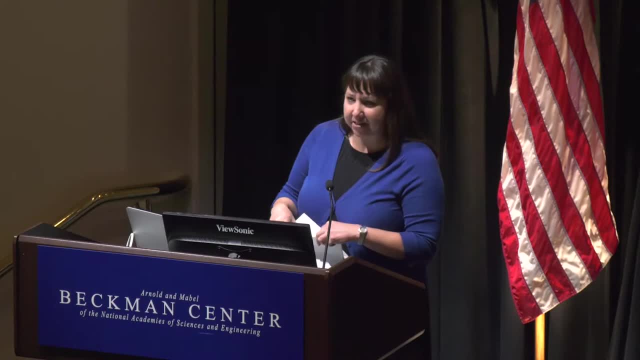 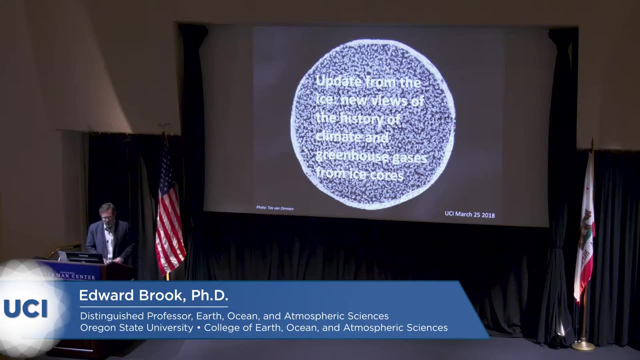 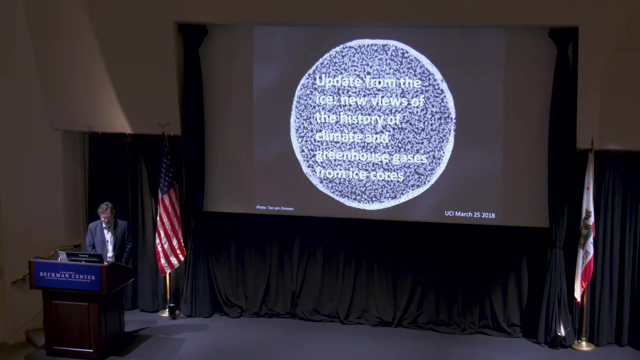 And, without further ado, I'd like to introduce Ed Brook to give the lecture. Thank you, Thanks very much for the introduction and for the invitation. It's a real pleasure to be here and it's really a pleasure to give a lecture named for Carolyn and Bill. 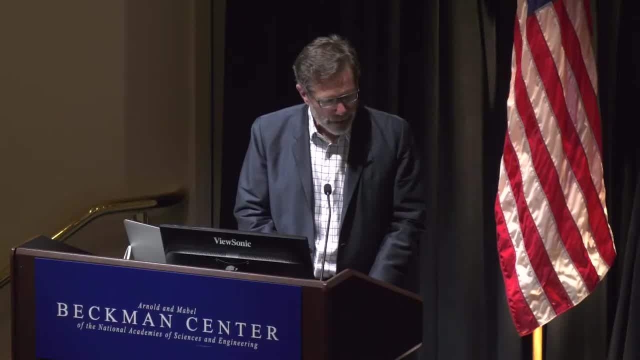 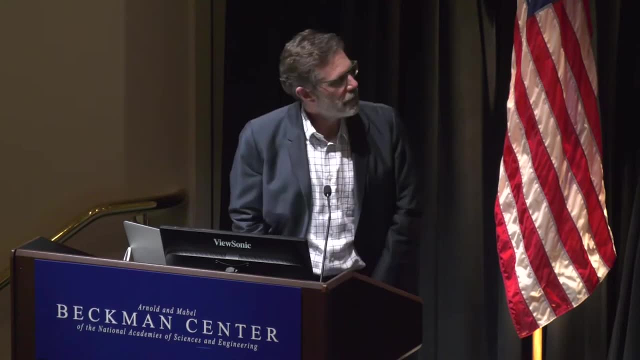 I've known Bill for quite some time. I'm very sorry that Carolyn is not here to have those conversations afterwards, But nonetheless it's great to be here. Every time I come here I learn a lot. This is a fantastic department. 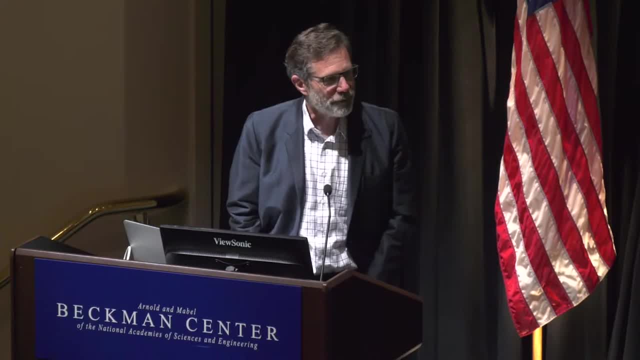 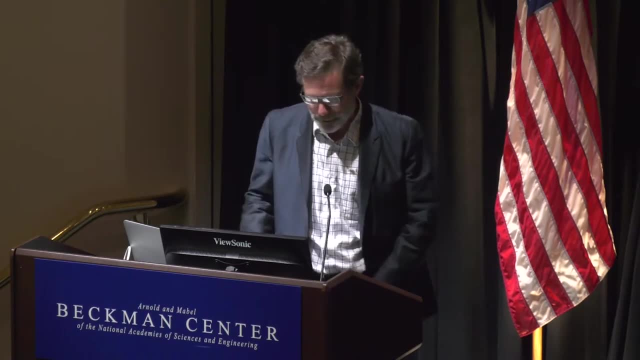 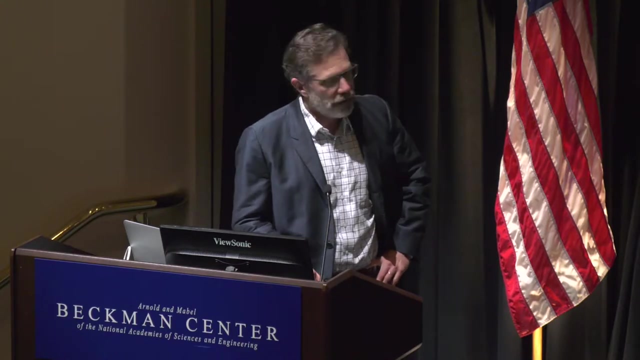 I think I got my PhD 25 years ago, so I couldn't have come here to study. But Woods Hole was OK, but it would have been fun to come here too. So what I would like to do today is kind of give. 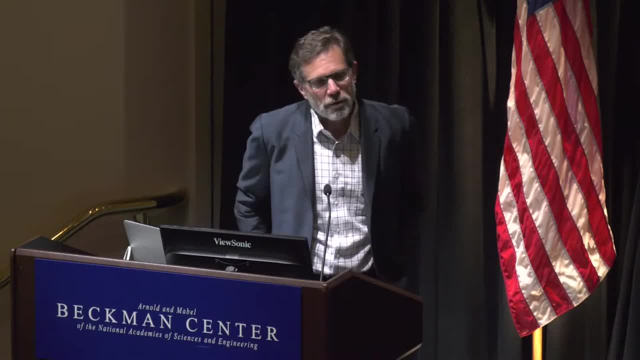 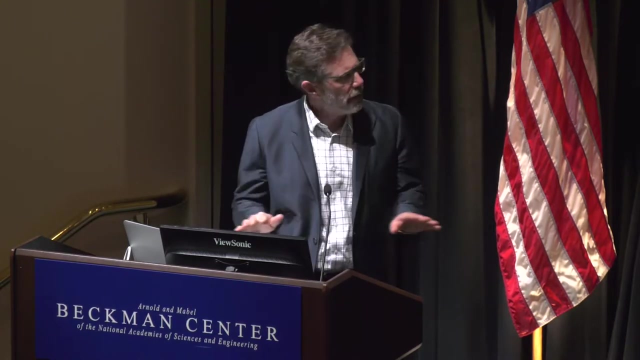 a broad discussion of some of the things we've learned about the history of greenhouse gases and climate from ice cores, sort of focusing on results that have come forward over the last 10 years or so. try to sort of keep it at a relatively basic level. 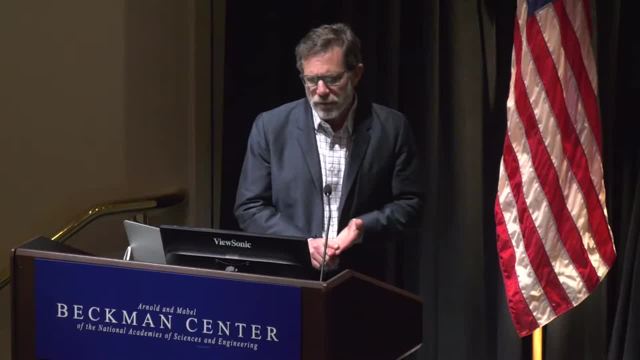 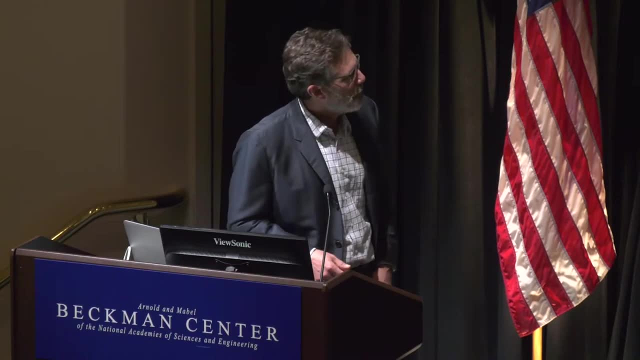 hopefully touch on some new things that people will be interested in. throw in a few of the more technical details now and then to keep Eric awake or some other people, And hopefully you'll get a sense of some of the things we're doing. 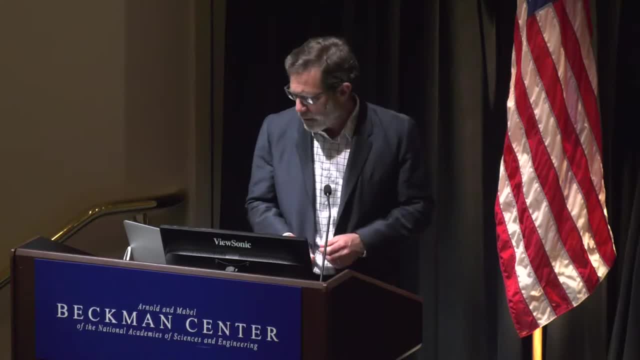 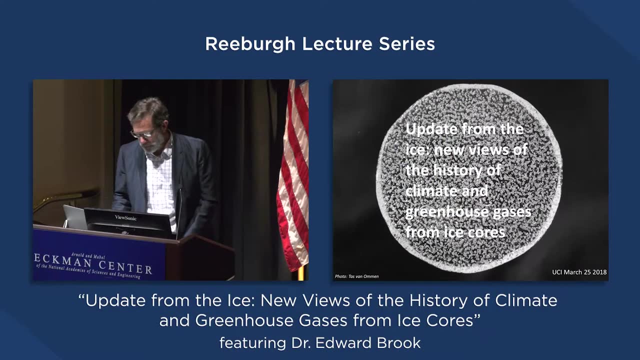 And I'll talk mostly about carbon dioxide and then talk in the beginning and then do some methane stuff near the end. So, to start with, a lot of people show pictures of their lab group when they first at the beginning of the talk. This is not my lab. 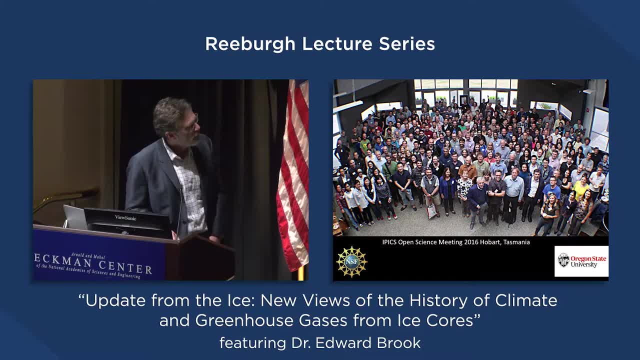 This is my lab group. This is most of the scientists who study ice cores in the world at a conference in 2016.. And I'm just showing this photograph to remind myself, to say that we, like many people, work on sort of big projects that take many people. 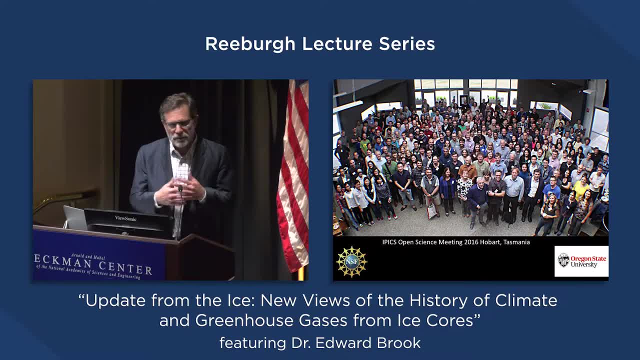 to accomplish. There are data in this talk from projects from all over the world. Can't thank all the folks, But I just wanted to emphasize the point that this is a scientific community. Not all scientific communities are friendly. This one actually is a very friendly scientific community. 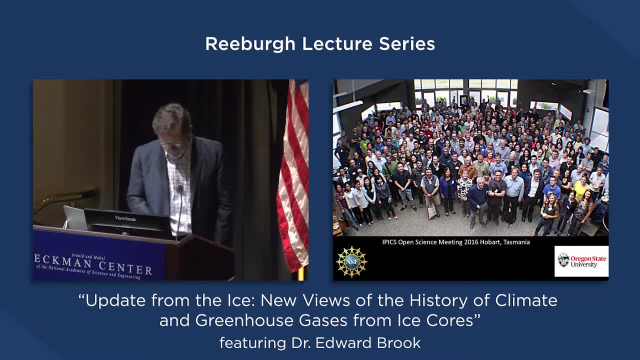 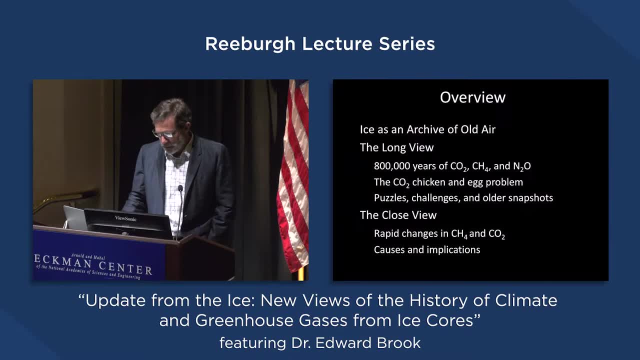 and part of the reason I enjoy working in there, And you could pick out your favorite ice core scientist if you look closely. So just an overview of what I'd like to talk about. First of all. just a little bit of the basics about why we can get air out of ice, how that works. 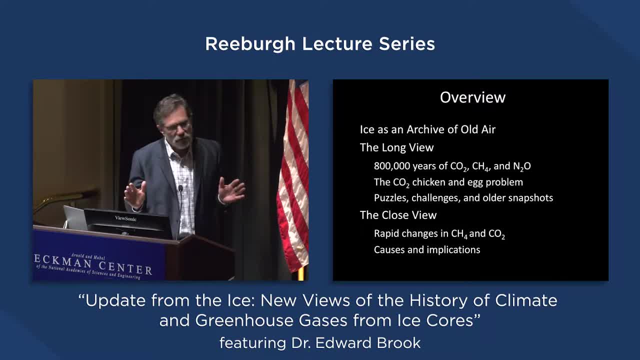 And then we'll take sort of the long view. talk about it. talk about the long records of greenhouse gases that cover 800,000 years. talk about one of the sort of vexing problems in this field that gets into the news now and then when we think about the reality. 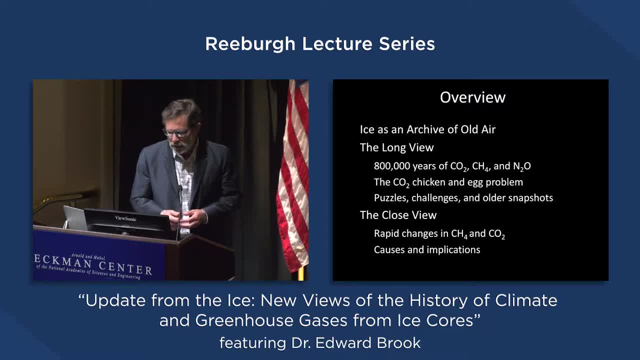 of climate change- that has to do with the timing of temperature and CO2 change, something we studied recently- And then say just a little bit about some of the puzzles and challenges that have come up in this work. And then I'll say a little bit about a new project that 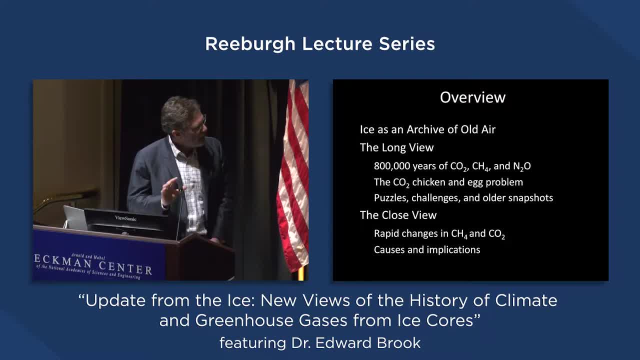 actually looks at older ice, And then we'll move on to talk about some of the things that Kathleen sort of alluded to: rapid changes in methane and CO2 and what might be causing them and what implications they have for what might be happening in the future. 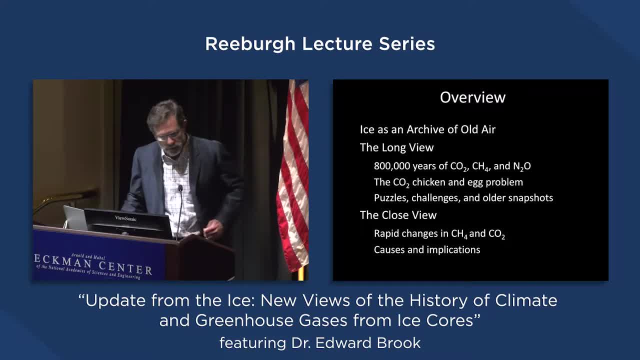 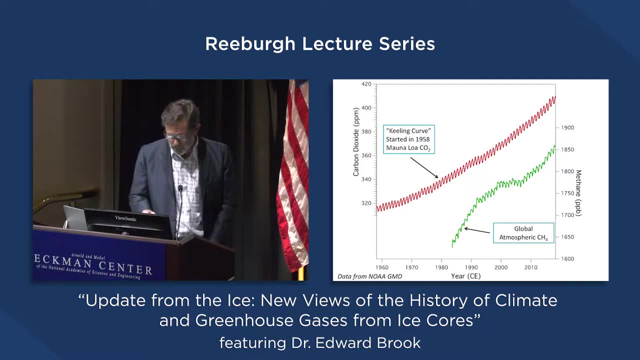 So that's where we're going. I may have to flip through a few things quickly to make it on time, but we'll see how it happens. Just to start with, to set the stage, something a lot of people in this room know a lot about- the increase. 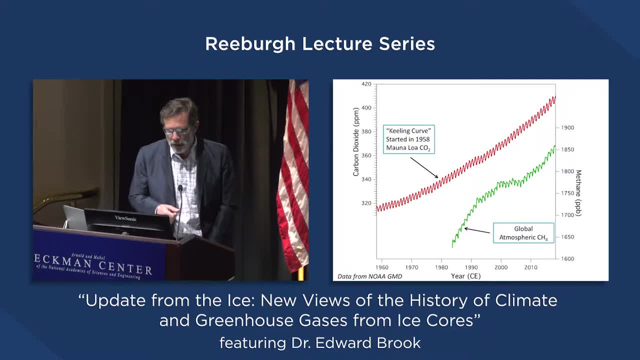 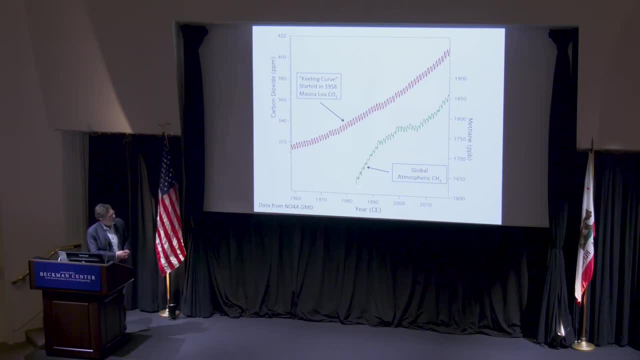 in atmospheric carbon dioxide in the modern atmosphere measured at Mauna Loa, the Keeling curve, and then also shown here in green measurements of atmospheric methane, also rising rapidly, And both of these curves also have had input from people here. 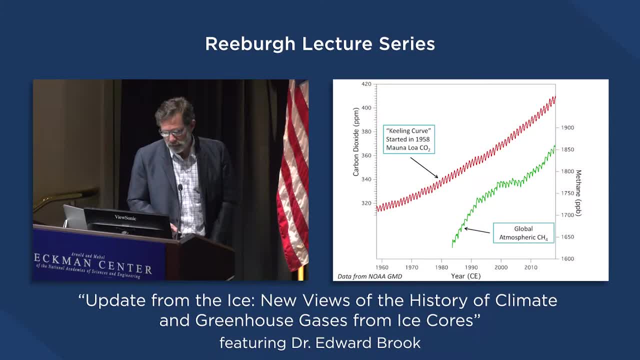 I believe The point of showing this is not to prove to you that CO2 and methane are rising- I think most people understand that- But to say that the direct measurements of these gases in the atmosphere in a systematic way only go back to really the late 1950s. 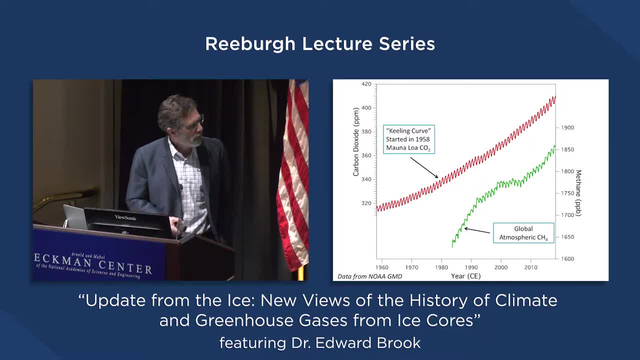 And to understand the atmosphere before this. while there are scattered measurements for earlier times, we really have to go to the ICE archive to get a detailed picture of how the atmosphere evolved. It turns out that around the time that Keeling was beginning this measurement program, 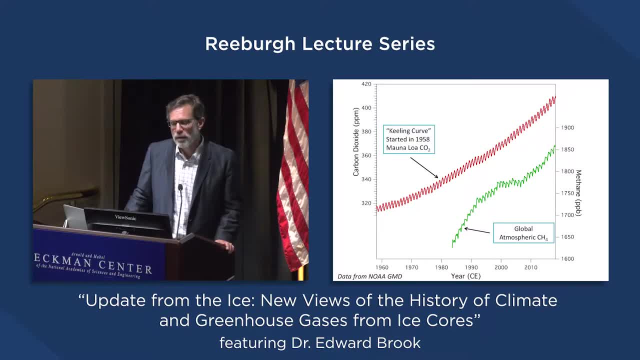 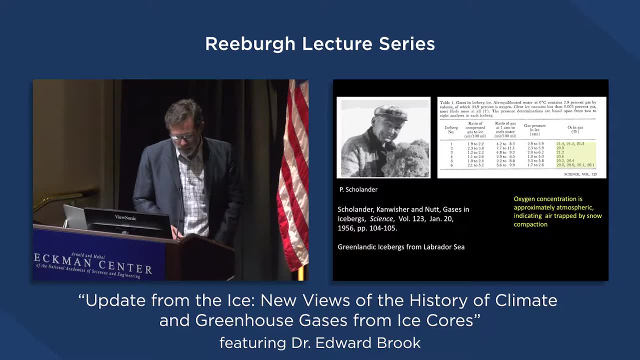 it was the same time that the people who started thinking about the ICE as a way of understanding the atmosphere, And so this gentleman, Per Schollander, who worked at a number of places, including Scripps Institution of Oceanography, thought about gases in ICE in the 1950s. 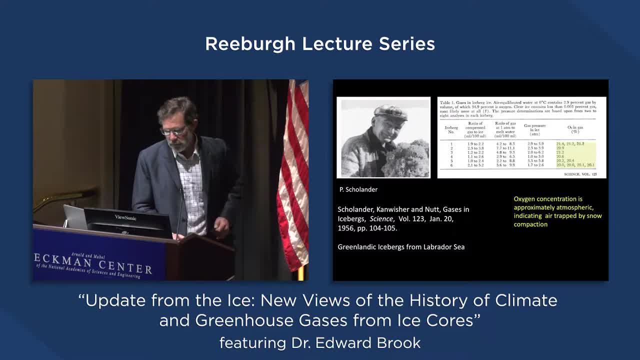 and recognized that it is possible that ICE would preserve a record of the atmosphere And they actually got on a boat and went out and collected ice bergs off in the Labrador Sea and measured gases in the ICE. And they couldn't measure trace gases at the time really. 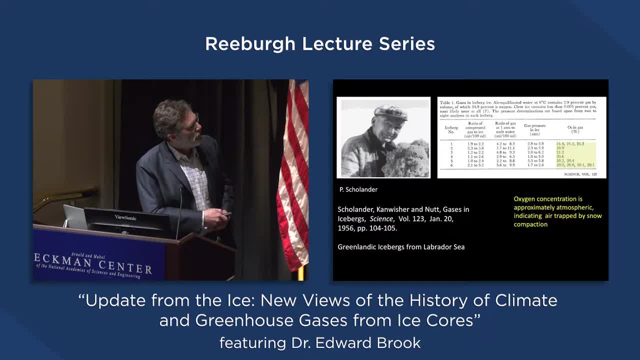 But this is a table from that paper And the point of the table was that the oxygen that they measured when they extracted the air was about the right number, around 20%, And he points out in this paper that this indicates that air was being trapped by the capacity. 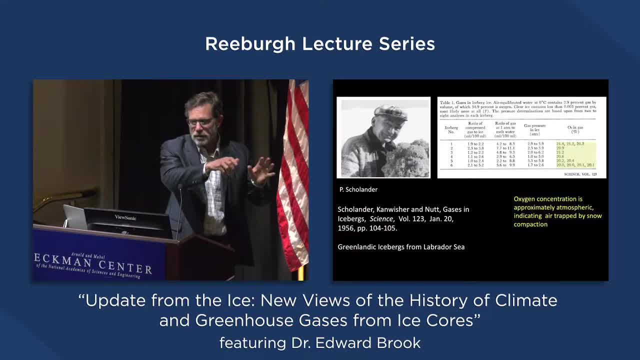 And the fact that the air was being trapped by the capacity was really interesting, And he also pointed out that the ice that was in the ICE was actually not a record of the ice. It was a record of the impact of snow on Greenland, And then the ice eventually flew into the ocean. 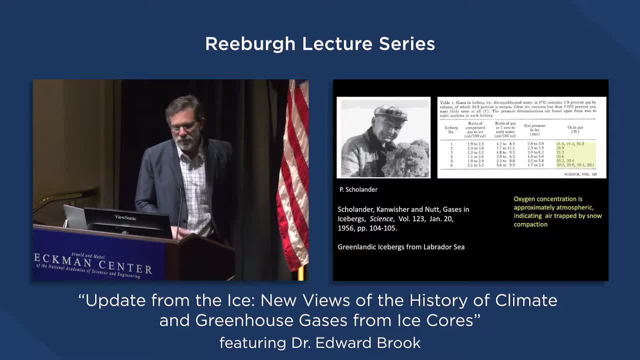 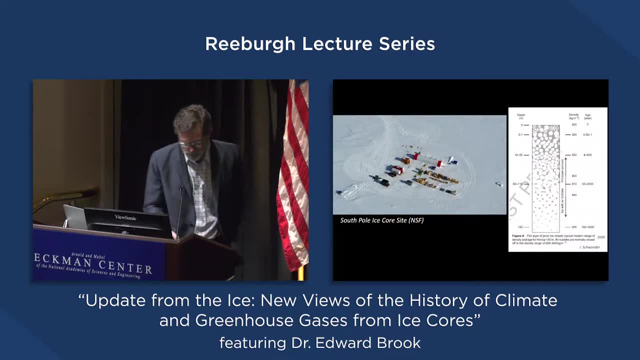 flowed into the ocean, And I think this is maybe not the first but one of the first suggestions that there might be a record of ancient air in ICE. Schollander went on to study the diffusion of gases in ICE and sort of really set the stage for the fact that we might be. 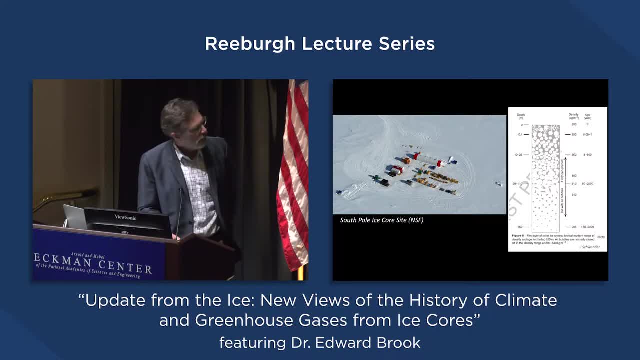 able to study this process, But this is a really interesting paper And the left hand is the ice core setting. The left hand photograph is this ice core drilling site at the South Pole. Several people here at UCI are involved in this project. 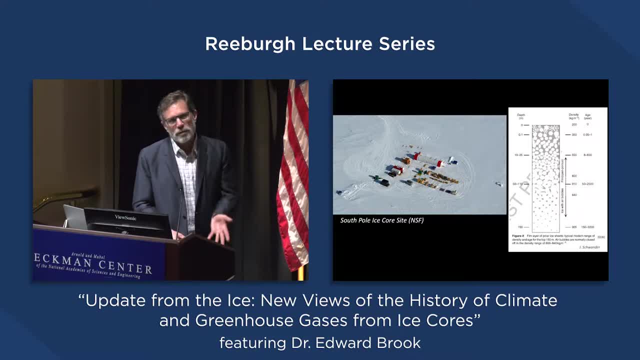 Just to sort of give you a picture of what the surface of the snow is like. the right hand side is a diagram of the fern, the unconsolidated snow pack at the upper parts of the ice sheets, And it is just a diagram to illustrate the fact. 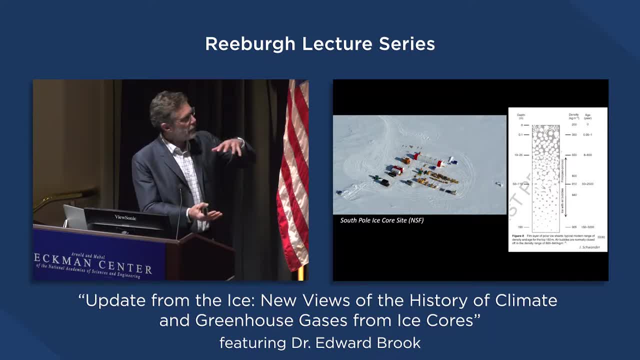 that air diffuses through the snow pack, gradually densifies, it compacts by the sliding of snow grains against each other and the recrystallization of snow grains, and ultimately traps the air as bubbles, and that's why we have a record of ancient air. 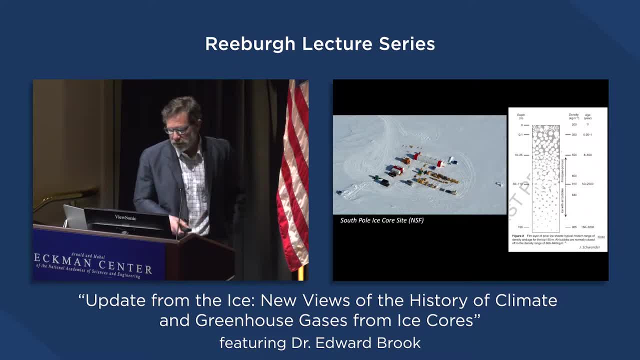 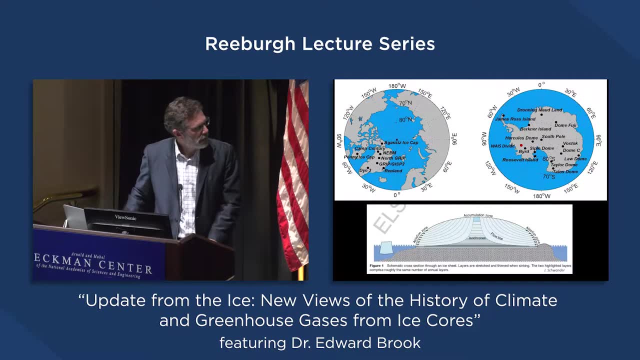 This also creates a problem related to the age of the air with respect to the age of the ice, which I'll come back to later. So, starting in the 1960s, various research groups around the world started drilling ice cores, both in Greenland and Antarctica. 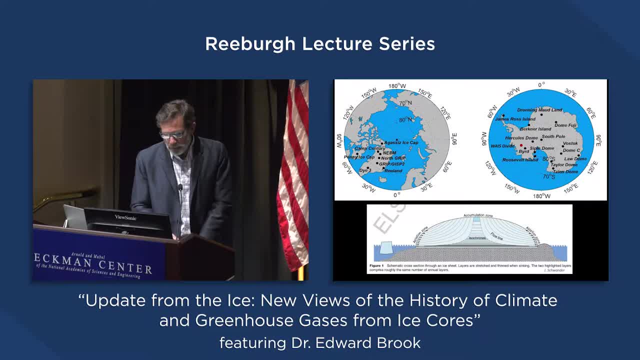 The major deep ice cores are shown on this map and there are cores in various places for various reasons, primarily because at different sites the snowfall rate is different and therefore both the detail that you can get from the records and the ultimate age of the records are different in different places, and typically we want to go to places. 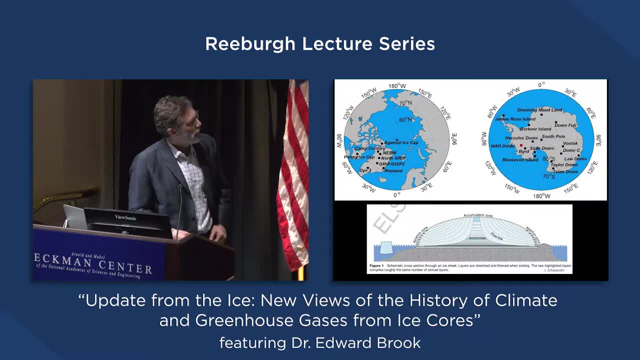 where the accumulation is relatively simple, where the ice flow is relatively simple and we can. We can easily interpret the stratigraphy as we go downward. I'm not going to say too much about ice core age scales in this talk, but we have a variety. 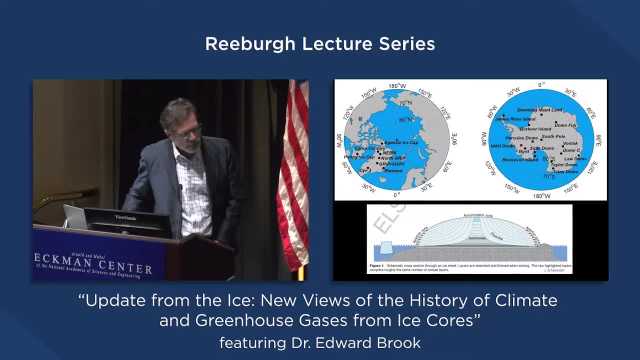 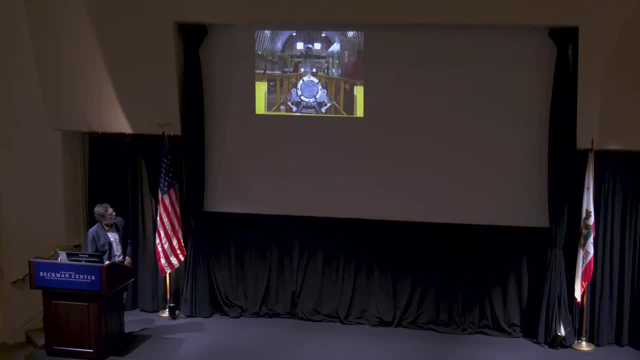 of ways of doing that. Like many kinds of science, there are lots of technical challenges for collecting ice cores. This is a photograph of the American One of the American ice core drills lying on its side. It's a sort of specialized engineering device. 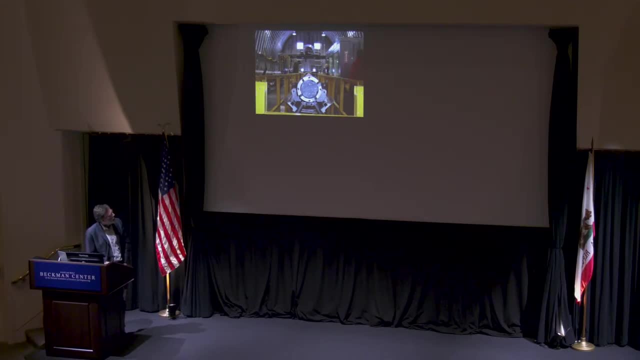 You can't go out and buy one And This is turned vertical- and I'll show you a movie of that in a minute- to actually operate it. You can see a core at the bottom And of course, we have to worry a lot about getting the ice back to the United States. 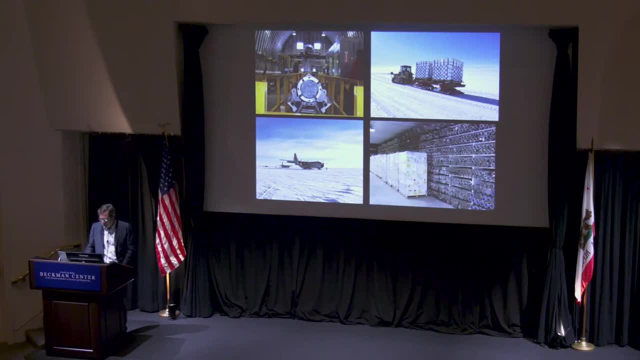 and safely and not melting it and then ultimately storing it. This is the National Ice Core Laboratory in Denver and I just show this photograph to make the point that these kinds of archives are extremely important, that all of the American ice core collection is here in Denver. 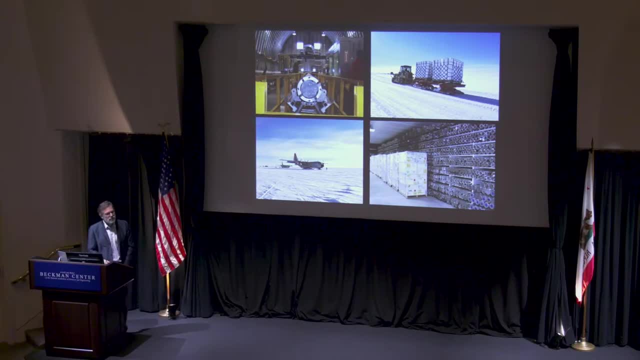 There are cores from the 1960s there that, in fact, my most cited paper comes from measurements we made on a core collected in 1967. So the support of archives like this is absolutely critical, And there's a story about this right now. 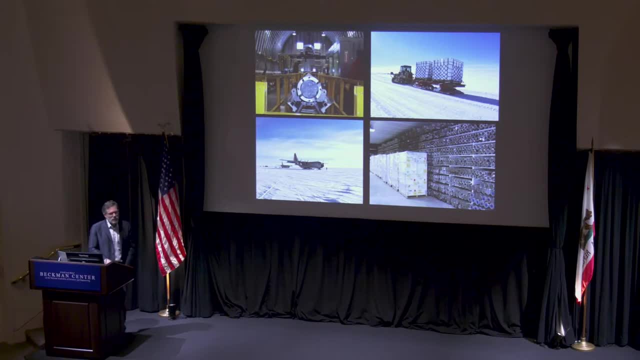 The cost of this archive is going up, apparently because the cost of warehouse space in Denver is increasing, and that's because of the marijuana industry. So You know, things are interesting sometimes. So, Thank you, I'm just going to show you a very short snippet of a movie that was actually entered into. 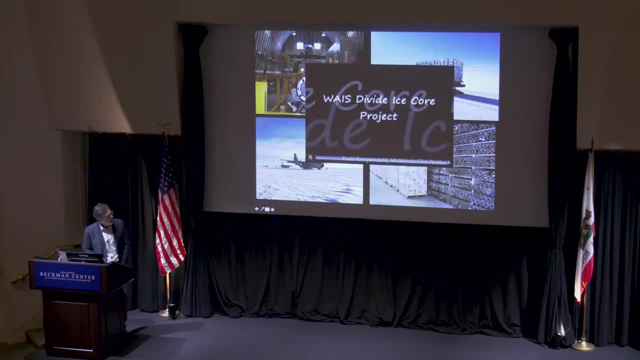 the McMurdo Station Film Festival. Some of you may have seen this, And there's a. What this person did is attach a camera to the top of the drill, So you're going to see the ice core drill lying on its side and it's going to tip up. 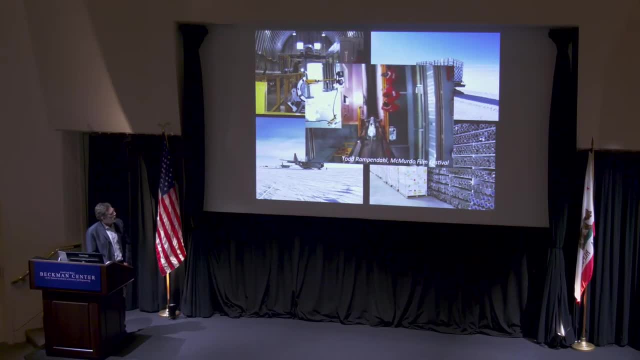 and it's going to go down into the hole and you'll see it hanging on its cable. It's a motorized device And so when it gets to the bottom it turns and drills into the ice, and then they pull it back up and bring the samples to the surface. 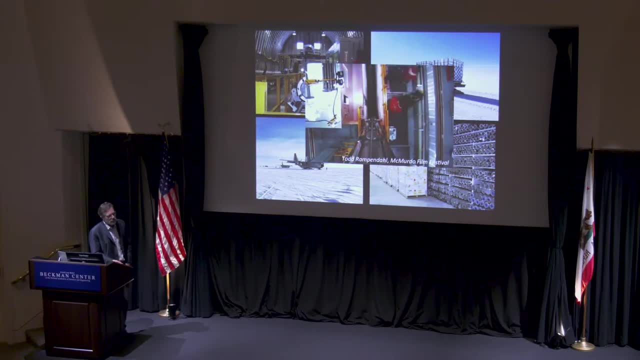 You have to do that over and over and over again, because you're going down 3,000 or plus meters in some cases. So there's music to this, but not serious enough for this audience, Anyway. so that's sort of the technology. There's quite a bit involved and of course this is way out in the middle of Antarctica, so You know we're quite grateful to the funding agencies for being able to do that. Of course, then when we get home, I'm also showing what is the stage and what I'd like. to do is talk a little bit about the work that we've done on two of the problems related to these sort of long-term cycles, And one of the problems is a fire. It's fairly simple to get at, and that is the timing of carbon dioxide and methane change. with respect to temperature, There's been a lot of sort of discussion, both in scientific literature and sort of leaking out into the popular media, about this chicken and egg problem, CO2 change before or after temperature on these sort of As you go from an ice age to a warm period, and what does that mean? Does it invalidate greenhouse gases that are important for climate? You hear things like that, And then I'll also just say a little bit about mechanisms of carbon dioxide change, and this is a much harder problem that lots and lots of people work on- just say a few things about. that, And to do that, I'm gonna introduce two different sort of newer archives of ice. One is something called the Waste Divide Ice Core in West Antarctica, a project that finished relatively recently and provided some new windows on On some of these problems, and I'm gonna talk about a fun project that we're working on. with a number of colleagues on a glacier in Antarctica where we can get old ice at the surface, And so we'll start off by talking about the Waste Divide Project. This is in West Antarctica. Waste stands for West Antarctic Ice. Sheet Divide is at the ice divide, where ice is flowing off in several directions. The ice core is located here. The reason to go here. The reason to go here. The reason to go here was that the snowfall rate is quite high and most Antarctic ice cores have relatively low snowfall rates, and that The reason that's a problem has to do with this gas trapping in the ice. So we talked about this fern layer and the fact that bubbles are trapped here while the air diffuses through the snowpack relatively quickly on timescales of about a decade. so air trapped at the base of the fern here is actually Is trapped at the base of the fern. It's actually quite a bit younger than the ice that surrounds it, and that age difference can be very, very old. This is a graph from 70,000 years ago to zero of this age difference, called delta age, for a variety of different ice cores. The ones up here are all from places where the snowfall rates are very low, and you can see that these numbers go from about 2,000 years up to about 4,000 or even 5,000 years, And you can see that these numbers go from about 2,000 years up to about 4,000 or even. 5,000 years, And you can see that these numbers go from about 2,000 years up to about 4,000 or even 5,000 years. Those numbers are big and they're uncertain and that creates an uncertainty when we want. to understand the age of changes in the gas phase relative to something that is in the ice that we're interested in, for example, isotopes that tell us about temperature change. So Antarctica is the place we want to go if we want to reconstruct carbon dioxide levels. because the ice is clean. but if we want to answer the chicken and egg problem, we need to be down in here. So we want to be down in here, where we have high snowfall rates and relatively low values of the parameter delta H, so that we can get a more accurate understanding of timing. So that's why we went to this site And, oops, wrong direction. The diagram on the right is a summary of what we found. This is data from a paper Discovered by Sean Marcotte, who is a postdoc in my group. The diagram comes from a summary article that's in press in Nature, And what it shows is carbon dioxide change from the waste divide, ice core, as well as a composite record of temperature change in Antarctica. This is actually the anomaly in the Antarctic: 18 oxygen to 16 oxygen ratio. but you can think of the pattern as a pattern of temperature change And if you look closely, starting at about a dozen years ago, this is the end of the ice age. CO2 starts to rise And it actually has several fits and starts. It doesn't rise monotonically. And you can also see, if you look closely, that the timing of temperature change in Antarctica actually matches the timing of CO2 change. It's very difficult to discern a lead or a lag between these two variables. This is important. This is important because previous work had suggested that carbon dioxide change actually lagged behind Antarctic temperature change by about 800 years And those data were from one of these cores where the gas age, ice age difference is very big and it was just difficult to constrain properly And they would agree with us now that this very, very synchronous behavior is really. the right answer. So Antarctic temperature and carbon dioxide are. I'm sorry, Carbon dioxide are essentially changing at the same time. Now you might ask: well okay, what does that actually mean? Maybe it tells us something about the greenhouse effect, but we're really interested in the global temperature if we want to be thinking about how global change works And global temperatures are harder to reconstruct. but the best sort of average reconstruction of global temperature by going all over the world and collecting all of the possible temperature indicators They could be obtained- Jeremy Schacken, in 2012, created this curve and when you compare these- and it's fair to make the comparison- actually CO2 starts to rise. Rises a little bit faster than global temperature. There's a little bit of a lead of CO2 over global temperature and that makes a lot of. sense and the system seems to be working the way we think it should. Why are Antarctic temperature and carbon dioxide coupled so tightly? That probably has something to do with more specific dynamics of the carbon cycle and ocean circulation, And the sort of dominant thinking these days is that the ventilation of the deep ocean around Antarctica. and changes in biological activity in the ocean around Antarctica are probably the reason why these things seem to be so coupled together And there's lots and lots of people trying to understand the details of that problem. Methane is hanging out up here waiting for us to talk about it. but it's also the case that the rise in methane happens almost exactly at the same time as the rise in CO2. It has these other sort of spiky patterns and we're going to come back to that later. So CO2 and temperature are pretty tightly coupled. For this transition. this is the last transition from a cold period to a warm period. We actually can't do this yet for the older ones because we don't have detailed ice cores like this. going back further, We trade off length for detail. But the evidence that we do have for older transitions would support this conclusion. Why- And you could say a little bit more about why- the global temperatures are sort of lagging behind the Antarctic temperature. This has to do with something called the bipolar seesaw. There's actually kind of an oscillation in heat between the northern and southern hemispheres that we infer from the ice core records. So when Antarctica starts to warm around 18,000 years ago, it's actually quite cold in the northern hemisphere. And this is probably due to the suppression of deep water formation in the north by freshwater processes, And that in the ice core records we can see this seesaw between the hemispheres And because Greenland is cold at this time, the average temperature of the Earth actually lags behind Antarctica. 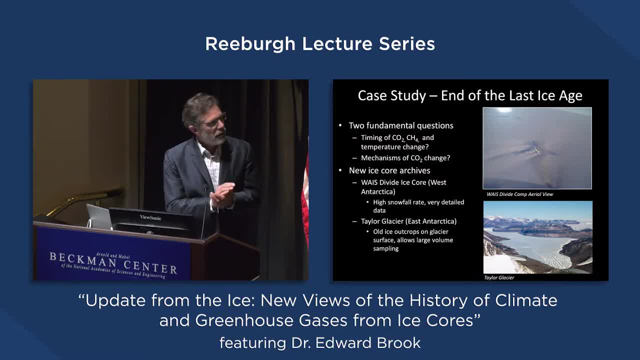 which is a little bit anomalously warm at this time. So the patterns that we see make a certain amount of sense, But one of the deeper questions I was alluding to is: why does CO2 change? Why does this feedback actually happen? 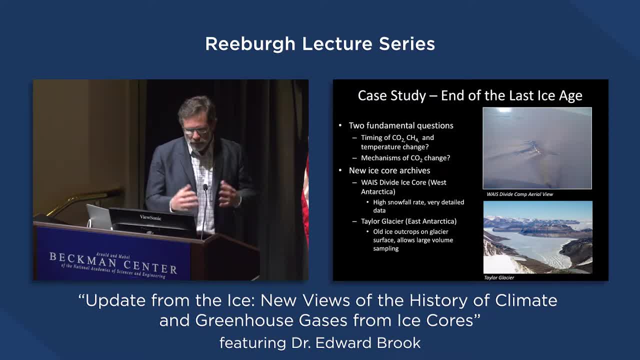 What are the mechanisms causing carbon dioxide to be involved in these long-term climate cycles? This is a tough problem. and it's a tough problem because, sort of illustrated by this carbon cycle diagram, the amount of carbon in the atmosphere is relatively small. 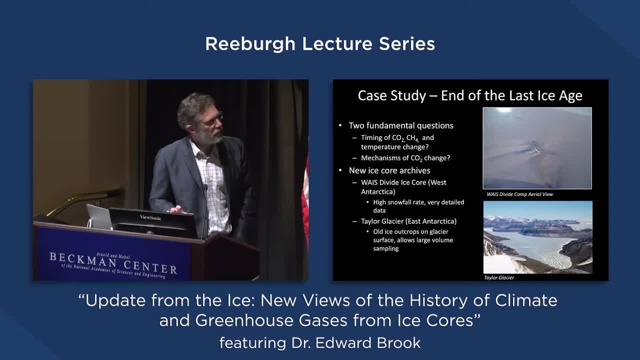 compared to all of the reservoirs of the carbon cycle, And what the atmospheric level really represents is the balance of all the fluxes in and out of the atmosphere, And we're asking to understand all of these from the geological record, and it's actually quite a difficult task.